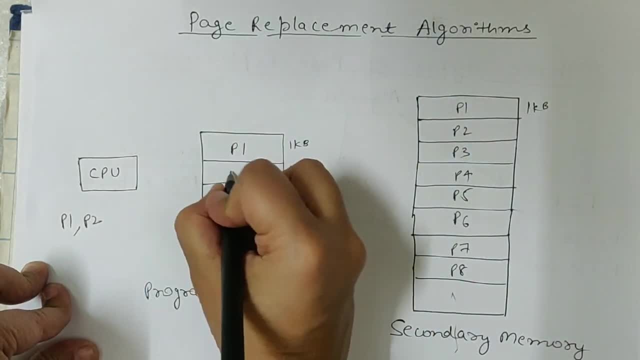 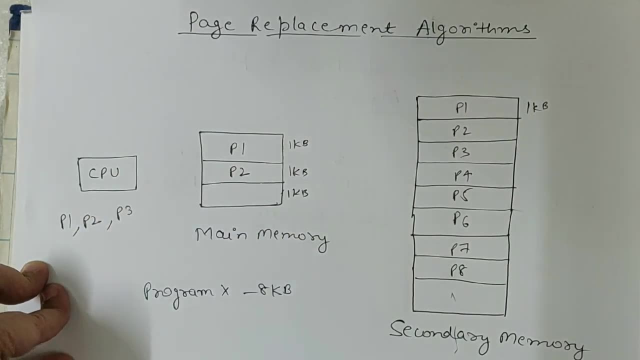 searches the main memory, it is not present. So it will bring that page in the main memory and then picks up and execute it. Now CPU wants page number 3.. Again, page fault occurs. It will bring the page number 3 to the main memory. Now execute the page number 3. CPU. 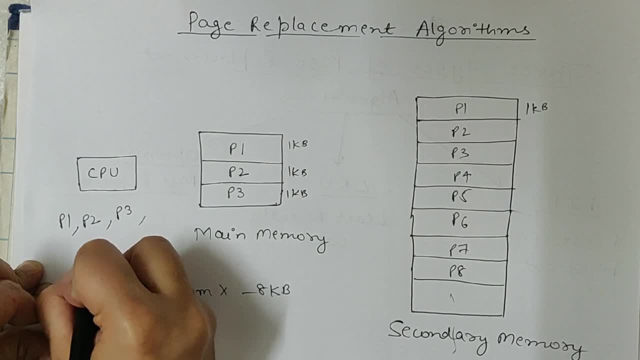 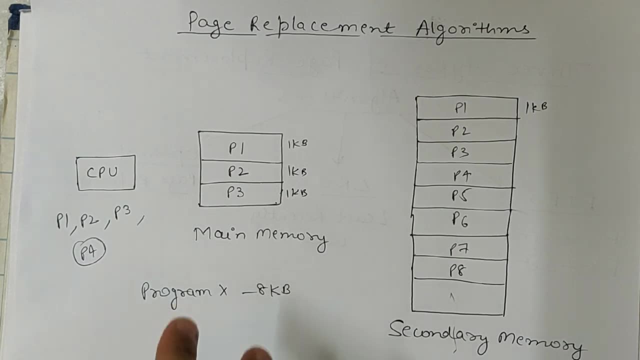 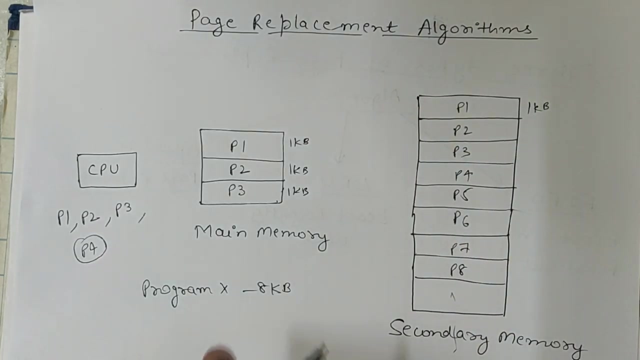 executes the page number 3.. Now CPU wants page number 4.. But now main memory is full, So page fault occurs and there is no space for page number 4.. So P1, P2, P3 from someone will have to go, because page fault has occurred And CPU 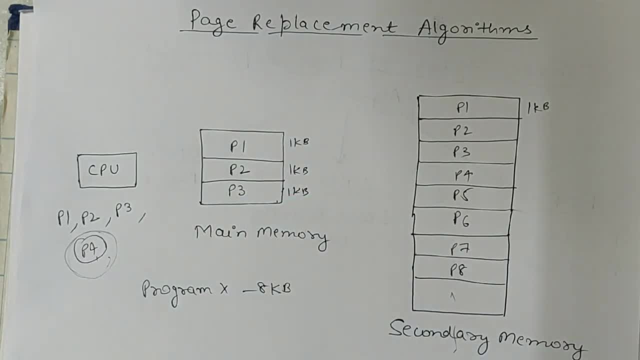 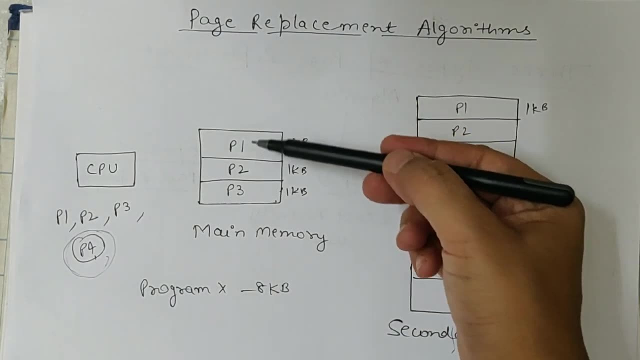 wants page number 4 now, And for page number 4 there is no free frame, So P4 will have to bring it from secondary memory to main memory. But main memory is full. So page number 1, 2 or 3 from these 3 someone will have to be replaced. 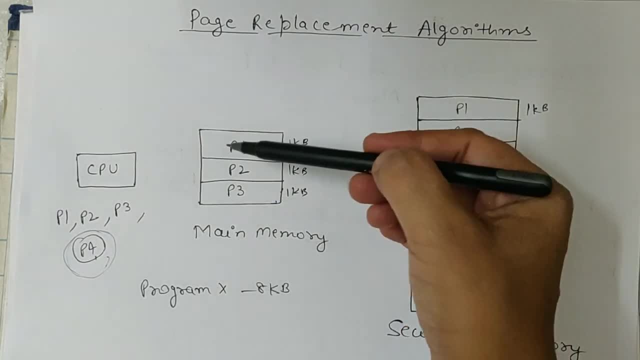 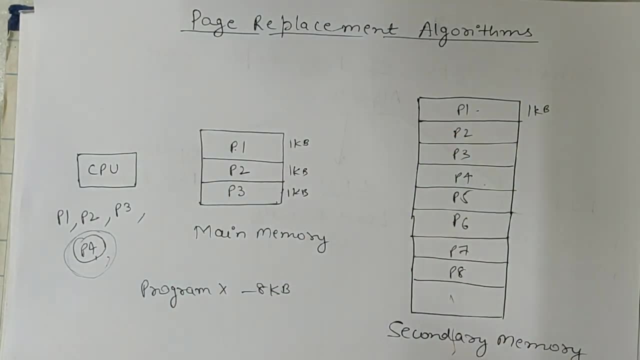 So now we can see how we can say that page number 1 can be removed so that page number 4 can be removed. Let's assume that I have sent the page number 1 to the secondary memory and bring page number 4.. So how can we make sure that the CPU will 자 две? 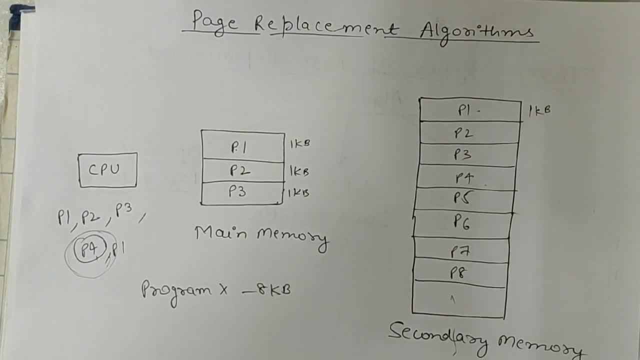 aley, listen to the requirement on the page no.1?. How can we decide the location of the power supply and the Mashableization present on the CCU and the main memory? How can we take theidirited decision Which page should go and which page shouldn't? 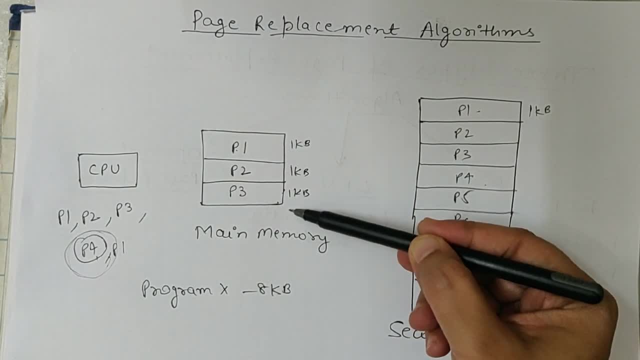 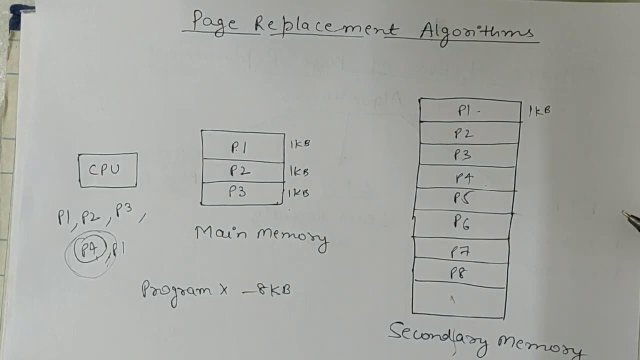 or page no.2 or page no.3. there should be some rule for that. we have made page replacement algorithms. we have total 3 algorithms which will decide which page will go back to the secondary memory. these are called page replacement algorithms. page replacement algorithms will decide. 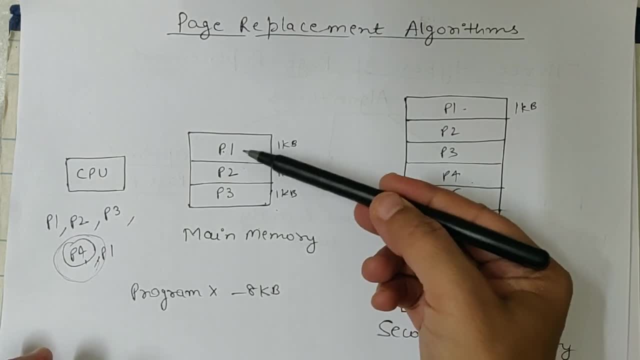 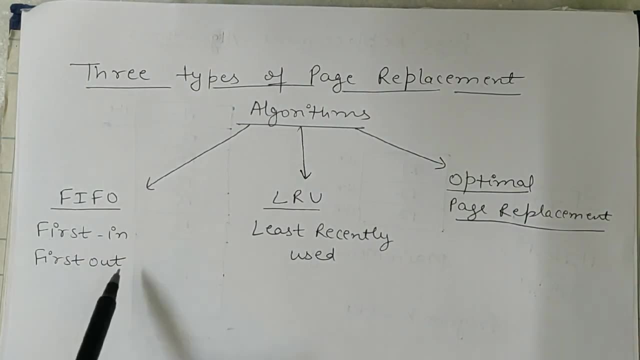 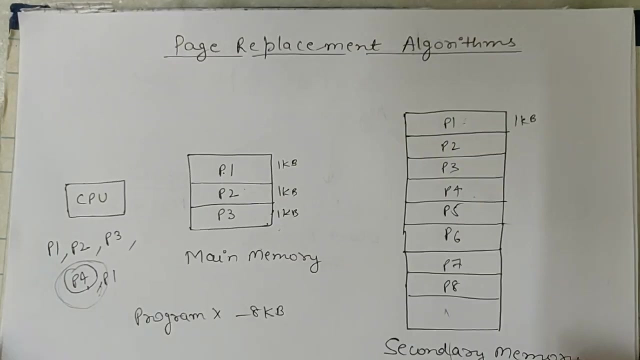 when main memory will be full, which page will be replaced. so we have 3 types of page replacement algorithms: FIFO: first in first out. first in first out means the page which came first replace that page. in this case we said P1 came first. if we are using FIFO algorithm, 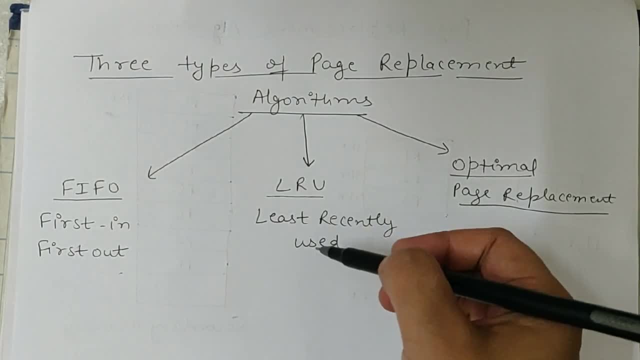 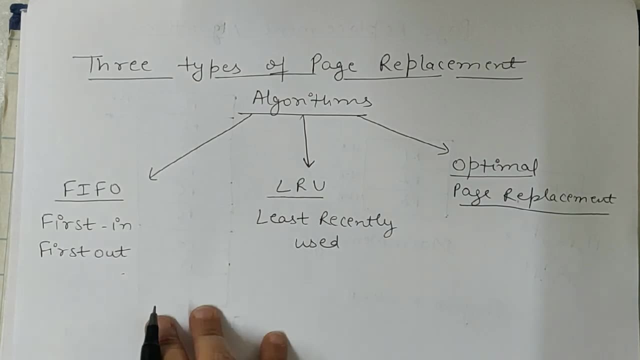 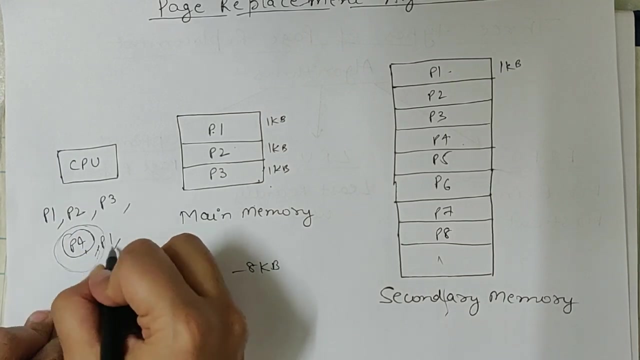 second algorithm is LRU. LRU stands for least recently used. it is saying that which was not used for long. send that page. how will we know this? suppose P1, P2, P3, P4. then CPU wants P2. then CPU wants P5, P6, P7, P8. 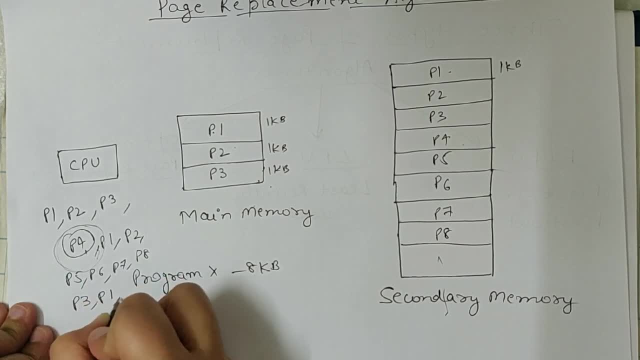 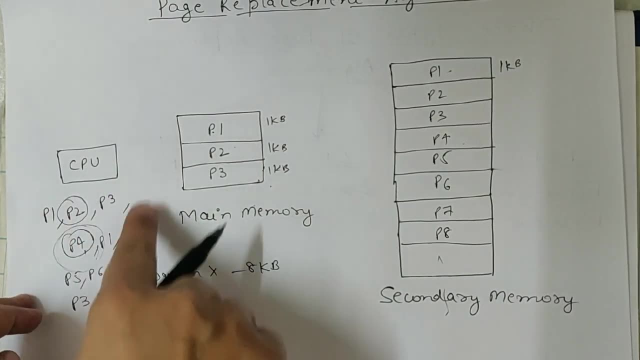 then again it wants P3, then again it wants P1, P4 and so on, but for a long time it did not give requirement of P2 CPU. for a long time in series it required whatever it wanted, but for a long time it did not show requirement of P2. 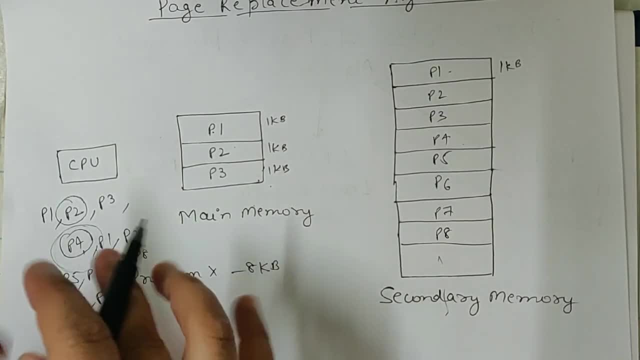 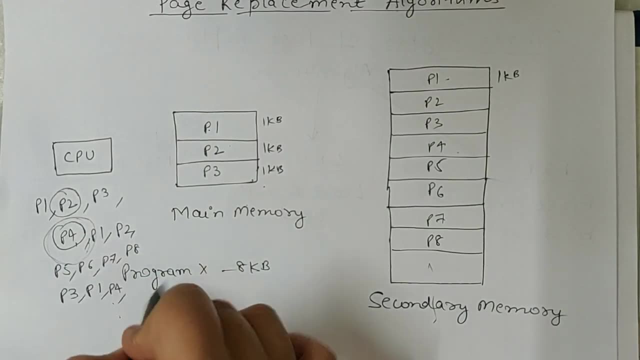 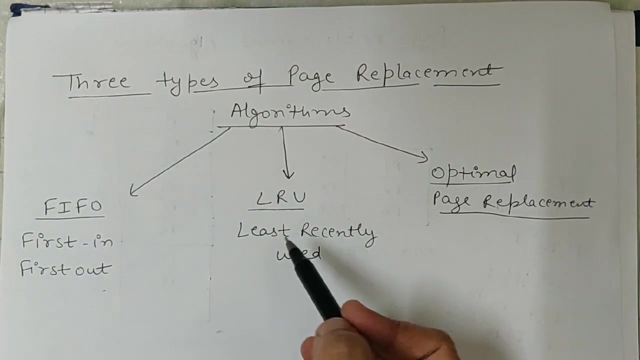 so for a long time. the page which CPU does not want to execute, replace that page. in this case, replace P2, because P2 has not been used for a long time. CPU has not demanded it for a long time, so replace the least recently used page. next is optimal page replacement algorithm. 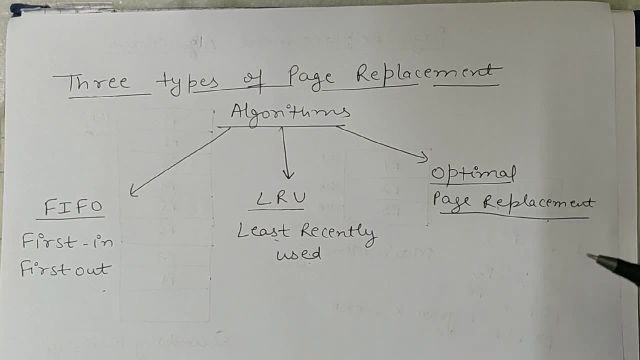 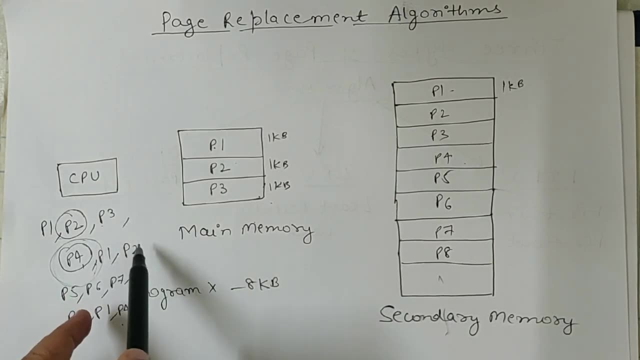 it says in future which is not going to be used for a long time. replace that page means we have to look ahead for a long time. P1, P2, P3, P4. P1, P4, P5, P6, P7, P8, P3, P1. 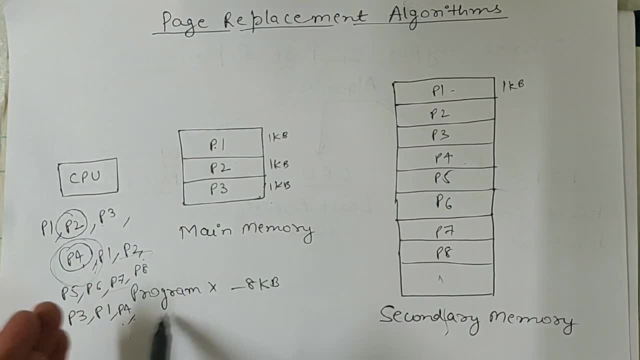 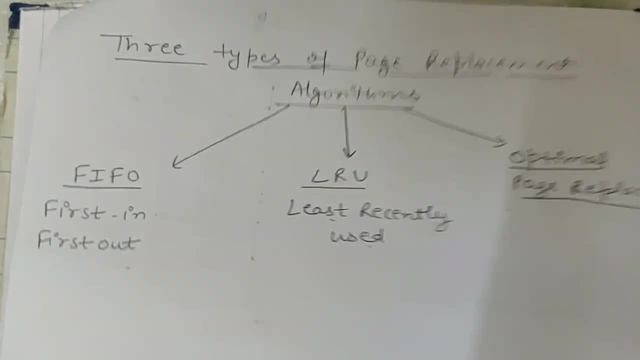 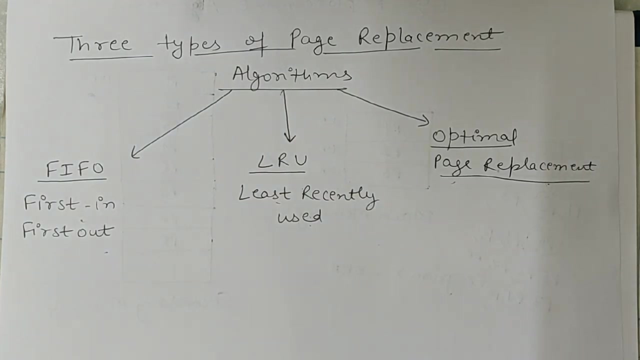 it means replace that page which is not going to be used for a long time. which is not going to be used for a long time, replace that page. so these are the three types of algorithms. first in, first out: LRU- optimal page replacement algorithm. next tutorial: I will discuss each of these. 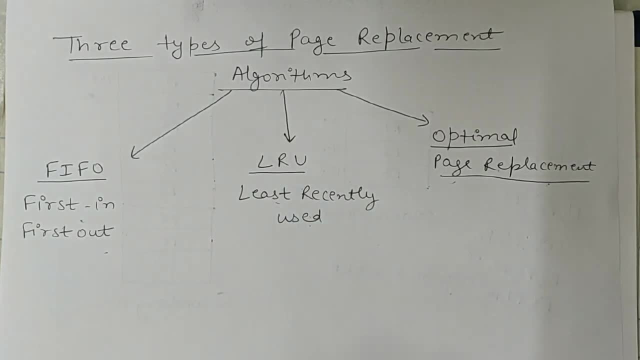 algorithms with the help of some numericals, so please watch my next video. I will explain all these three in separate videos. ok, so watch my next three videos about FIFO, LRU and optimal page replacement algorithms. thank you so much, everyone, and I hope this overview of page replacement algorithm clears now. 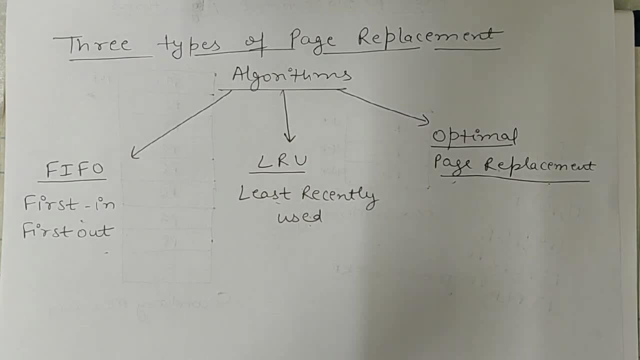 so please like and subscribe everyone. see you in next video. thank you so much.